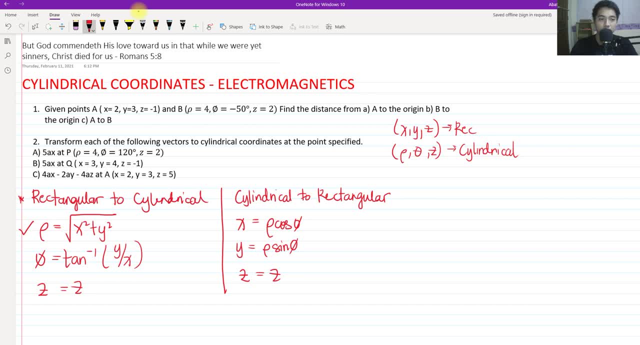 Of course the values of x, y, z must be given in order for us to convert it into cylindrical. And then we have the phi equals the arc tan of the y all over x and the z's are the same. Okay, just copy the z. So if we wish to convert from cylindrical coordinates phi, 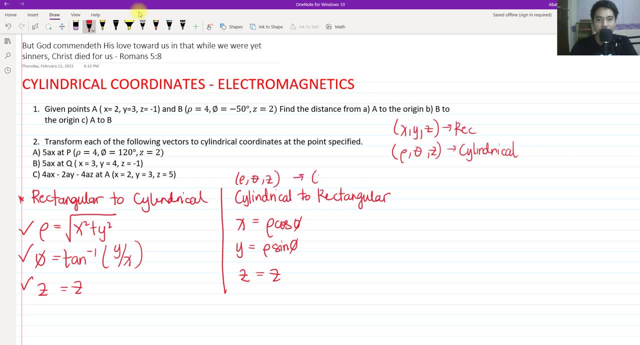 Theta and z to x, y, z. Okay, we need to use this following formula: So to get x, that's simply phi cosine of rho. I mean rho cosine of phi. This should be phi. I'm talking about phi, not theta. Okay, so sorry for that. So we have: this is rho and this is phi. 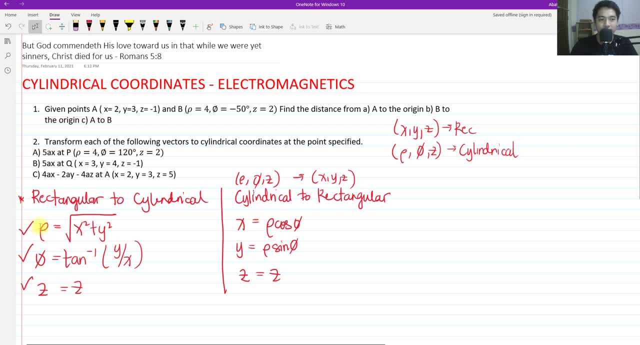 Okay, This one, just like the notation in physics, density, it's called rho and this is phi. So we have rho, cosine of phi, for x And then for y, we have rho, sine of phi, And then, as I have said a while ago, z's are the same. 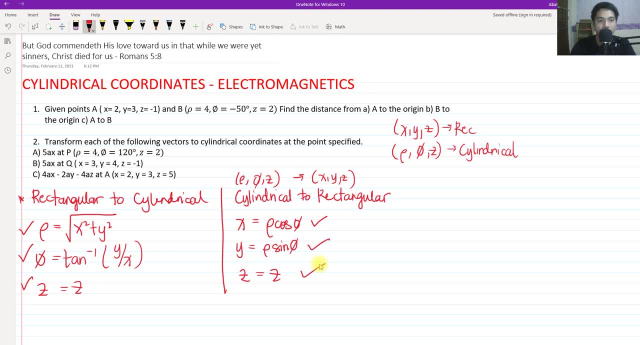 So that is the formula that we're going to use, So let's try to solve some problems. So, number one: given points A, we have x equals 2, y equals 3, z equals negative 1.. And B, we have the rho equals 4.. 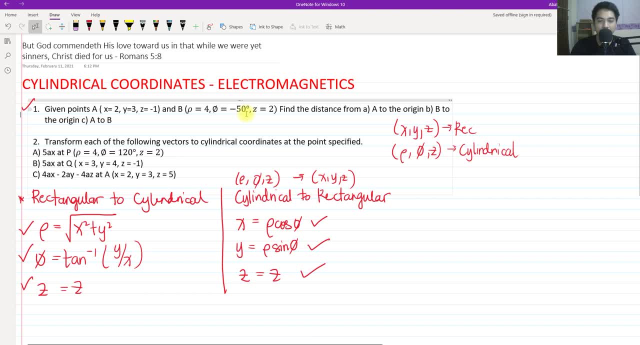 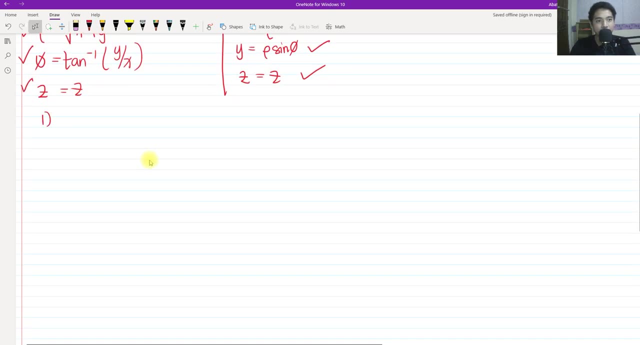 And then we have the phi equals negative 50 degrees, We have the z as 2. Find the distance from A- A to the origin. So what's the distance of the vector A to the origin? So for number one, we need to find the distance, okay, the vector of A to the origin. 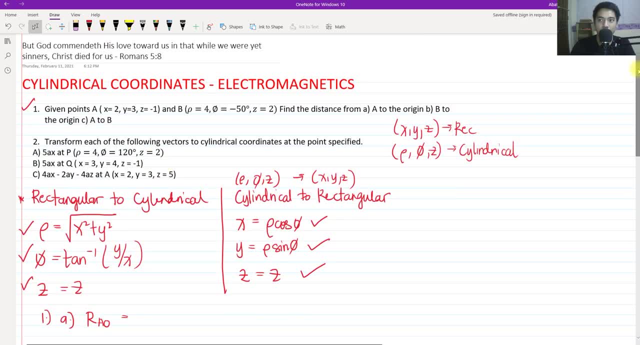 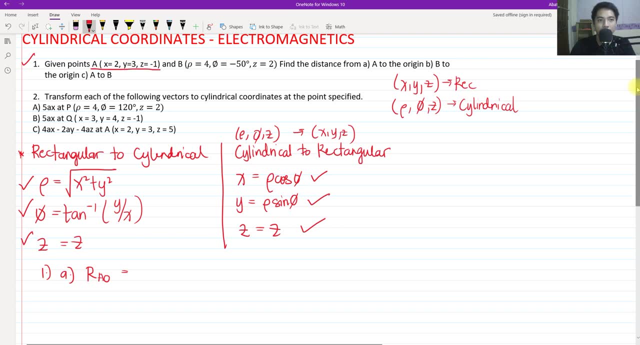 So our terminal point is the origin. So what are we going to do is still: First we have to find a vector from point A to the origin. So in that is, we know that. So the origin has coordinate 0, 0, 0. 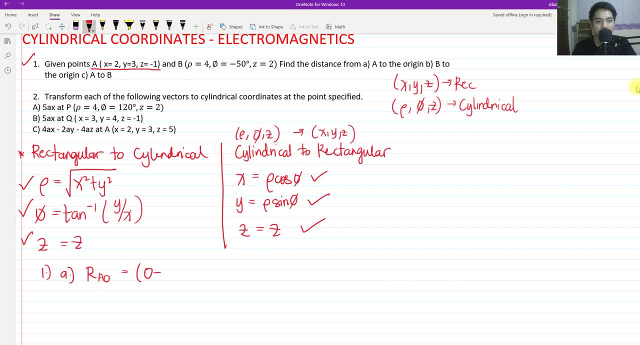 So that is our terminal point. So we have 0 minus the x component of the initial point, which is 2.. Then we have ax, Then we have plus 0 minus 3 for the y, Then we have plus. We have 0 minus negative 1 of z. okay, 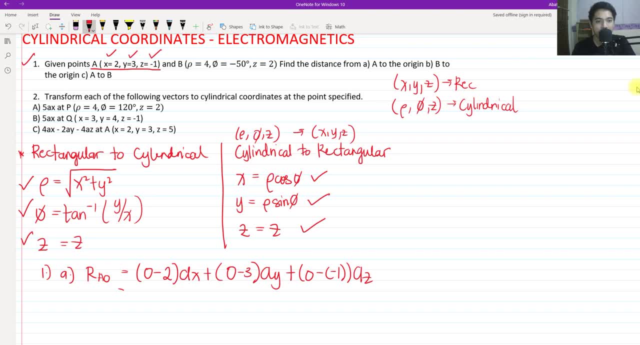 So that is what I'm trying to say. So we have negative 2ax minus 3ay plus a's of z, because minus times negative would be plus, Negative times negative would be plus. So in order for us, this is the vector, okay. 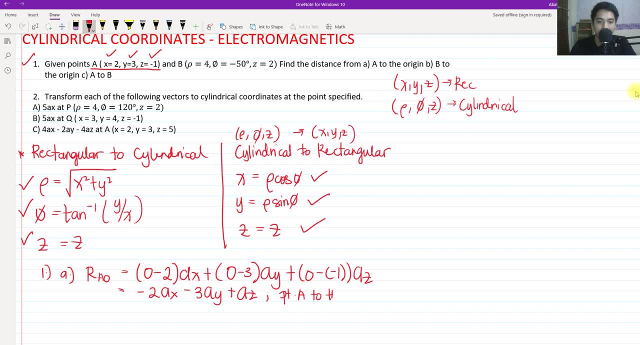 from point A to the origin. Okay, So if we wish to know the distance of this point A to the origin, okay, we simply get the magnitude. Okay, So what would be the magnitude? That's the distance, That's the length of our vector, negative 2 squared. 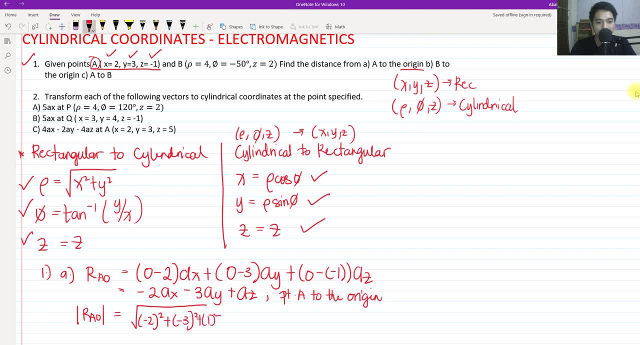 plus negative: 3 squared plus 1 squared. okay, So this would be squared. Let me just rewrite: So that would be what Square root of 14.. Or in terms of three decimals, so we have 3.742, okay. 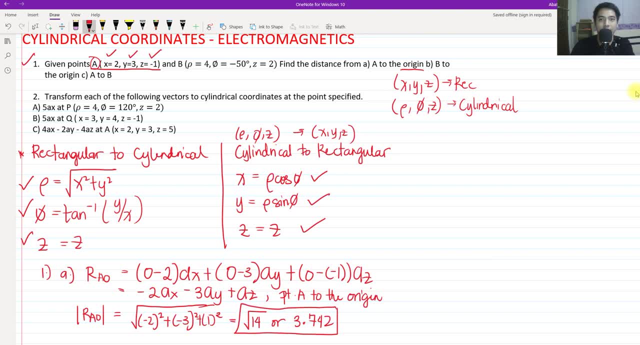 So that must be our answer for letter A, for number one. So check So you see, if we are asked to find the distance of a certain point to the origin, it's much better to use what Rectangular coordinates. okay, So letter B: 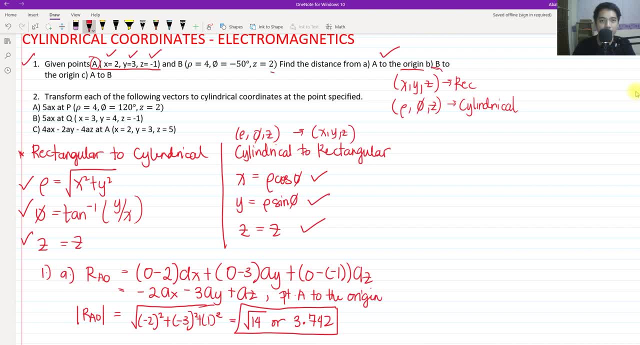 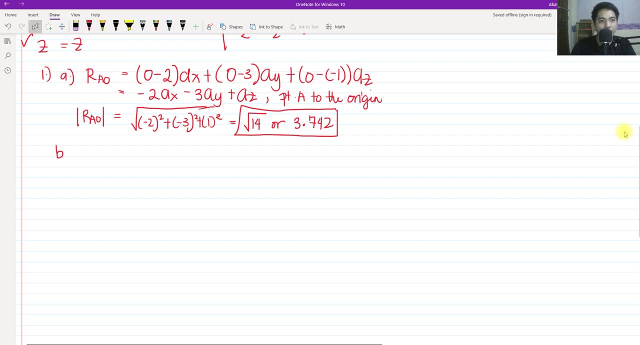 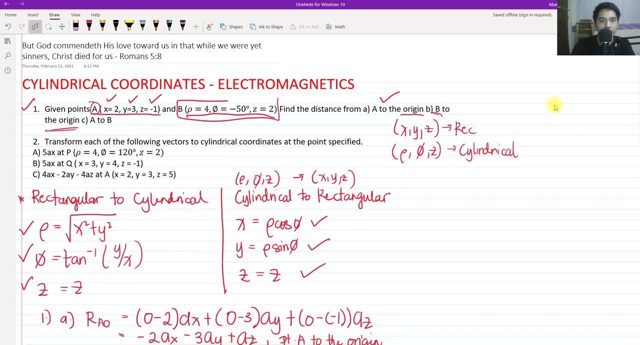 Find the distance from B point B- This is the point B in terms of cylindrical- to the origin. So, as I have said, it's more convenient to actually convert first the cylindrical point- okay, into what? Into rectangular point, and then get the magnitude of it, okay. 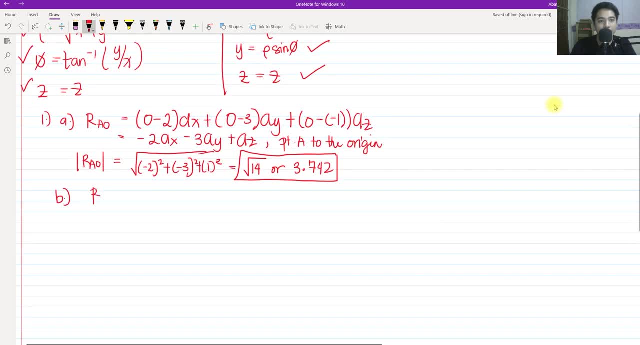 So we are going to get the point B is actually rho equals 4, and then we have phi equals negative 50. This is negative 50, and then we have z equals 2.. So we're going to convert this into rectangular. Take note that your calculator should be in terms of degree. 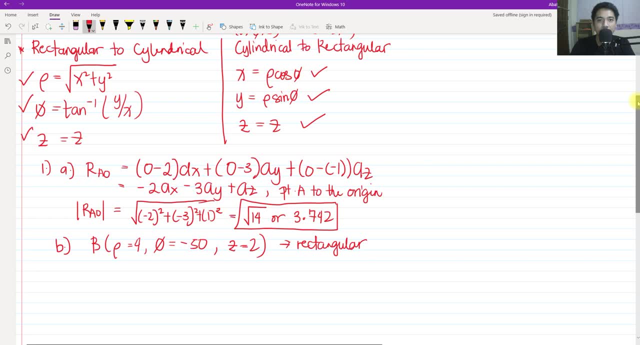 when you are converting these values. So we have cylindrical to rectangular, We're going to use this following formula: okay, We're going to use the following formula: So to get x, we have rho cosine of phi. So that is, 4 cosine of negative 50. 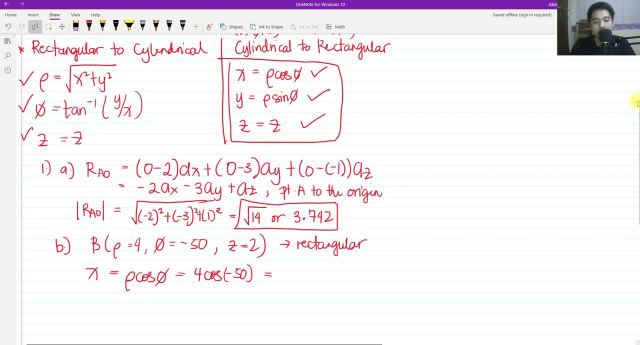 Okay, So that is 4 cosine of negative 50.. So our answer, if we calculate it in our calculator in three decimals, so that must be 2.571.. So we have y, we have rho sine of phi, We have 4 sine. 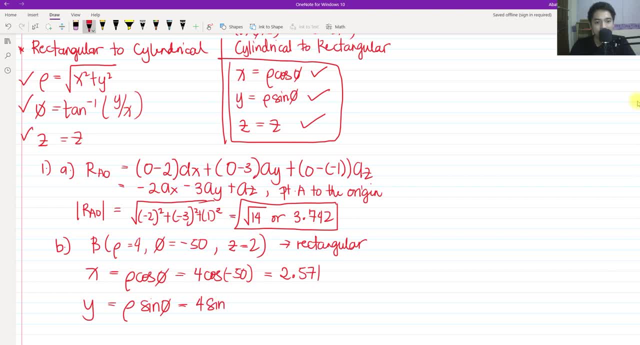 So we're just going to change the cosine into sine of negative 50, and that must be negative 3.064.. So this is our x, this is our 4.. So z equals only to z, which is actually 2.. 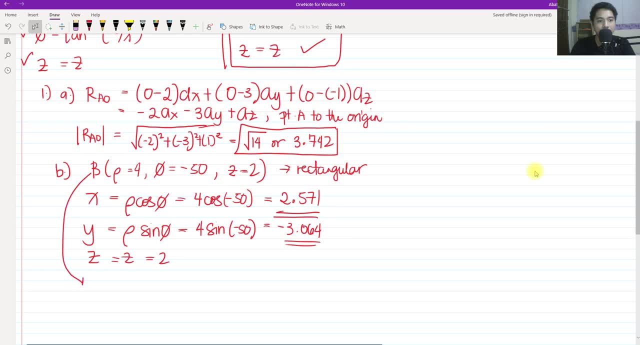 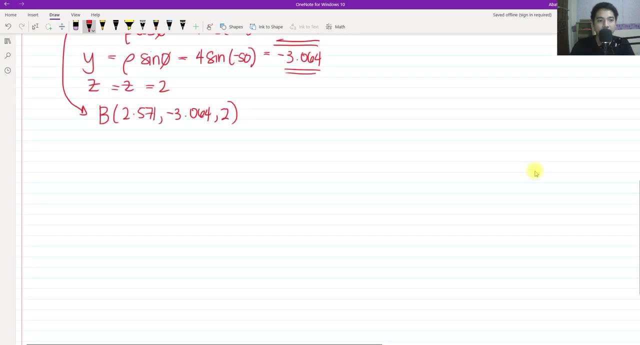 Therefore the coordinates of this point B, in terms of rectangular coordinates, that is 2.571,, then we have negative 3.064, and then we have 2.. So we are asked to find the distance of dot point to the origin. 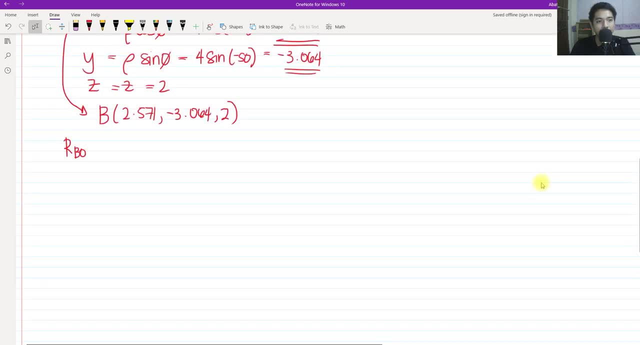 So again we have to get the vector rbo. From point b to point 3, to point b e, we have to find the distance of that point to the origin. So again we have to get the vector rbo. So again we have to get the vector rbo. 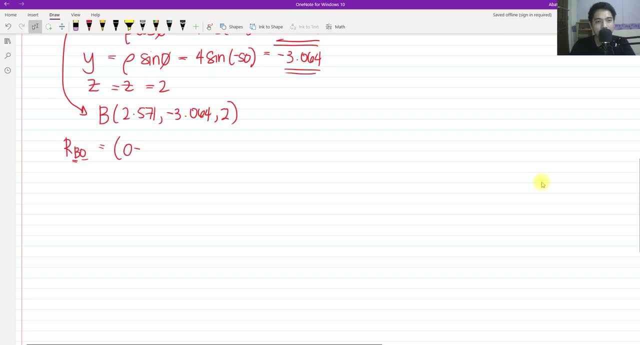 point b to the origin. so the origin is 0 minus 2.571 ax. then we have plus 0 minus the negative 3.064 a sub y. and then we have plus 0 minus 2 a sub c, so we have negative 2.571 ax. okay, plus. 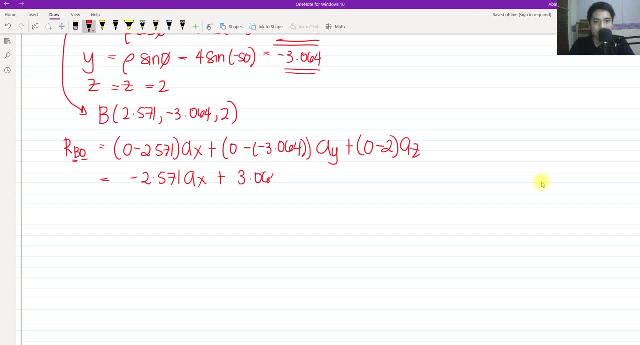 this is negative times negative. that becomes plus 3.064 ay, minus 2 a sub c. now this is the vector, okay, stretching from the point b to the origin. so how do we get the distance of that point to the origin? just get the resultant or the magnitude. so we have negative 2.571 squared. 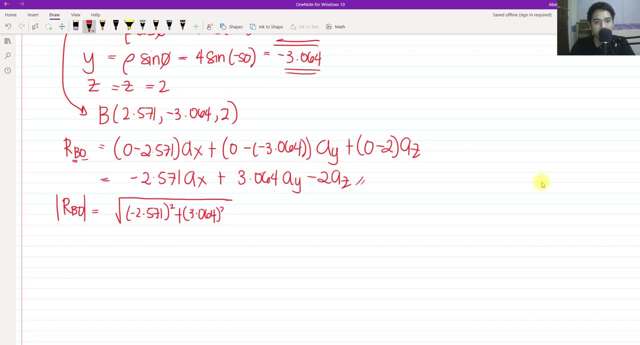 plus we have 3.064 squared. then we have plus negative 2 squared. so the answer in four decimal- or three decimals i mean that should be 4.472. so that's the distance from the point b to the origin. okay, just like what we. 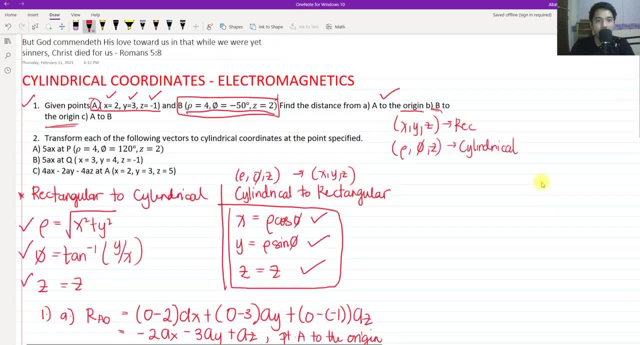 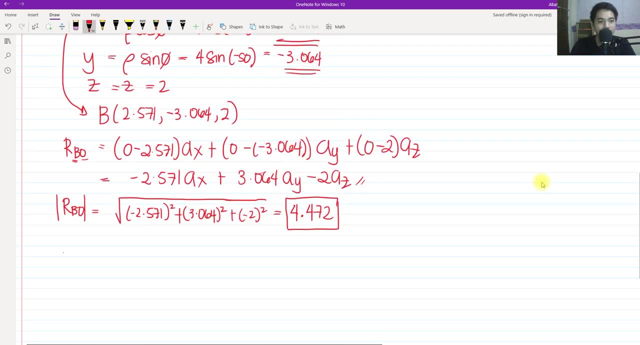 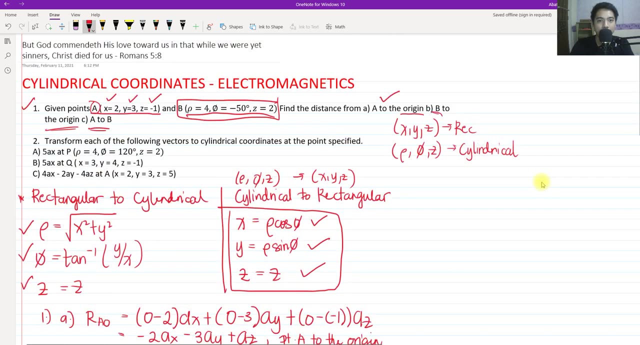 did on the first one, okay. so the last question for number one is the distance from a to b. so, since we have what? since we have both in terms of rectangular, this is point b, okay, and this is, uh, point a, okay. we have x, 2, y, 3, j, sub equals 1, so we 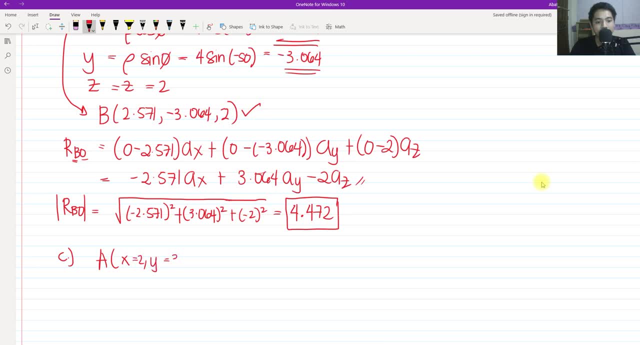 have x equals 2, y equals 3, and then we have j equals negative 1- if i'm not mistaken, that is negative 1 and point b in terms of rectangular. so we have 2.571 minus negative 3.064. and then we have: 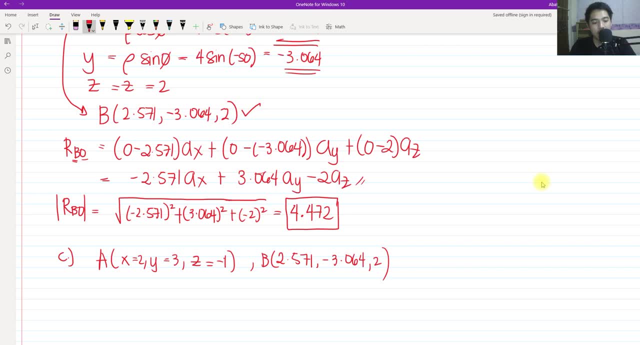 2. so the distance from a to b, okay, is actually what? oh, actually, we can use the distance formula. so, but first, that is still the same, we get the, the vector from a to b. so we have 2.571 minus 2. okay, for the x component, plus, we have 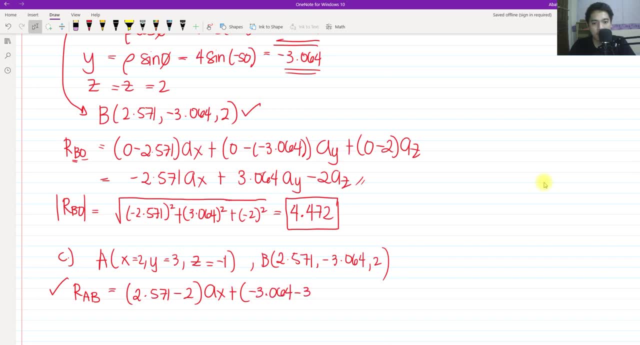 negative: 3.064. zero, six, four minus three for the y component. okay, so that should be our y component. and then plus we have two minus negative one for the a sub. say so terminal, terminal point, minus the initial point, in this case we have ab. so we have two minus negative one. so be careful with the sign. and 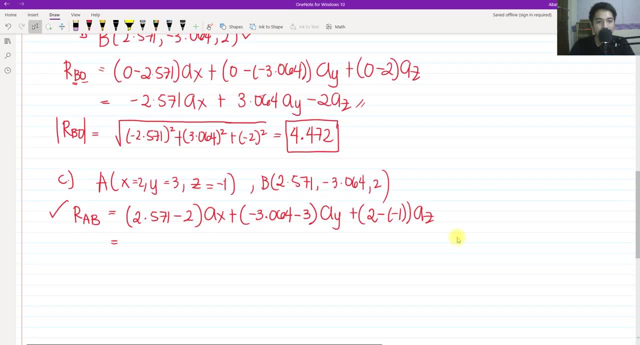 direction of the uh initial point to the final point. so we have 0.571 ax, we have negative 6.064, ay. then we have plus 3a sub say so this is the vector stretching from uh points a to b. so to get the distance between them we simply get the magnitude. okay, so we have 0.571 squared. 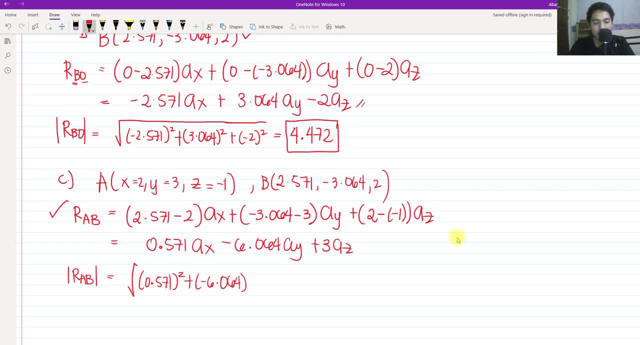 plus negative, negative: 6.064. we have squared plus, we have 3 squared, okay, and if we get the magnitude of that, that would be 6.79. so that is the distance of point a and point p. so let's go now to number two. let me just copy the problem number two. 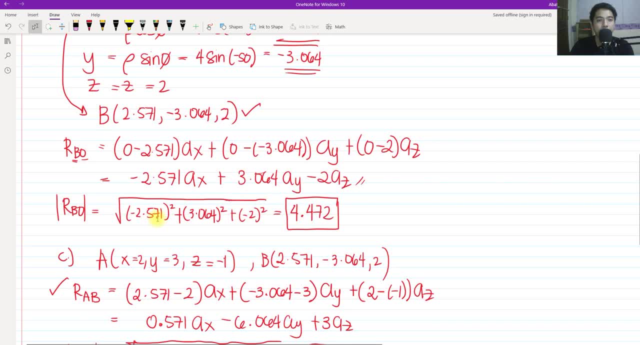 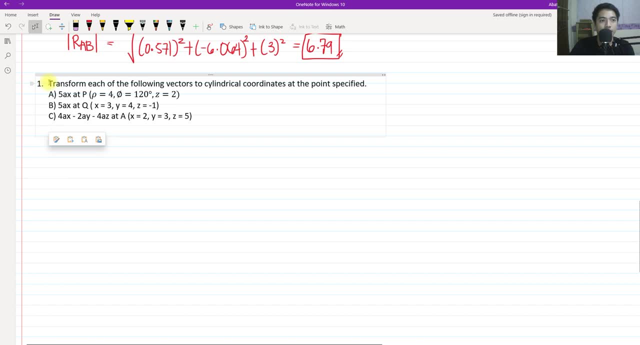 so that we'll be having a copy below. oops, okay, so in in number two: okay, we have to transform each the following vectors to cylindrical coordinates at this point, at the point specified: okay, so we are going to get the uh 5ax. at point p, we're going to transform: 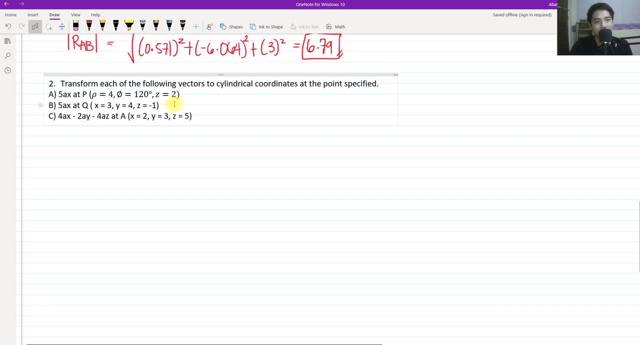 each of the following vectors to cylindrical coordinates at the point specified. so we have a 5ax vector. we are going to transform it into cylindrical coordinate at the point given: p, q and a. so for what are we going to do here is to take note, okay, of the important relationship. 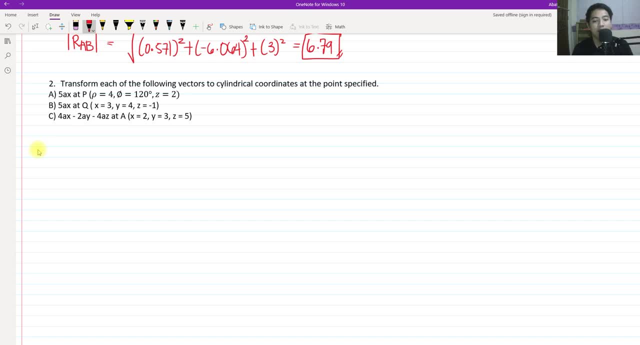 of the dot products between the rectangular and the cylindrical. so we have a table, we're getting the dot product. it's very important to memorize this actually, or familiarize yourself. so we have, for example, we have the, a component or row component for the cylindrical, and then we have 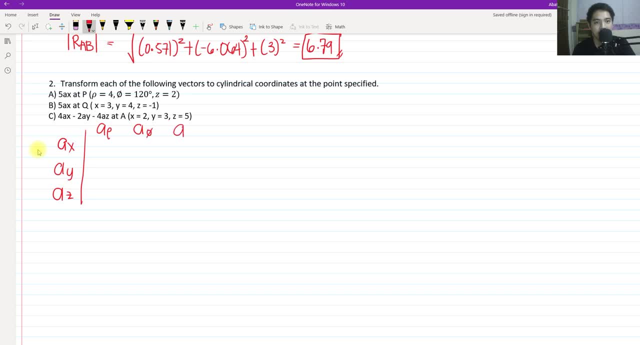 the phi component for cylindrical and then we have a sub c. so what are we going to do is that if we wish to get the cylindrical coordinates at a point specified, we have to remember the dot products. so this would be the dot product, and then we have the cylindrical, and then we have the 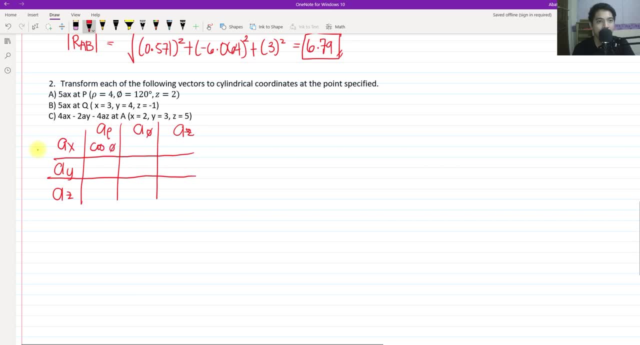 cosine of phi. okay, let me just rewrite this cosine of phi, negative sine of phi. then we have zero, zero and one. we have sine of phi, we have cosine of phi and then we have zero, zero, one. so what's the purpose of this? so for number letter a: okay, we are going to transform. 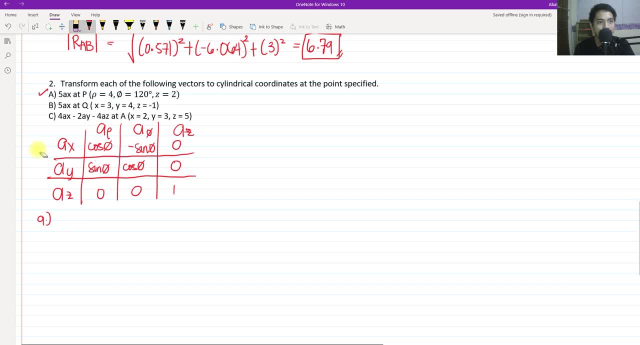 the vector five, a x at the point what? at the point p, which is a cylindrical coordinate. so we have row four, we have phi equals 120 degrees- okay, and we have z equals two. so we're going to transform that vector at the point specified. so we're going to use the dot product. so this is important. 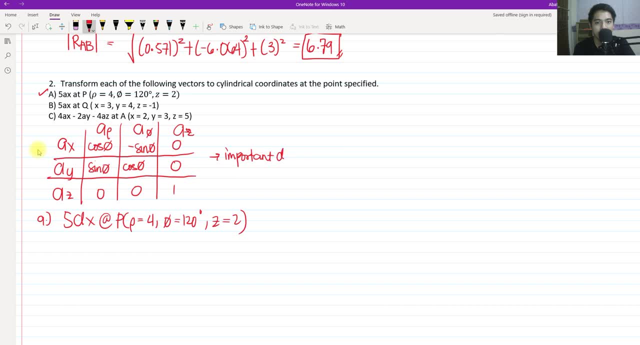 dot products: dot products when we are trying to get or transform a vector at a point specified. okay, important dot products for rect and cylindrical- rectangular and cylindrical. okay. so in order for us to answer this, let me just rewrite this: this should be five a x. okay. so what are we going to do? is we're going? 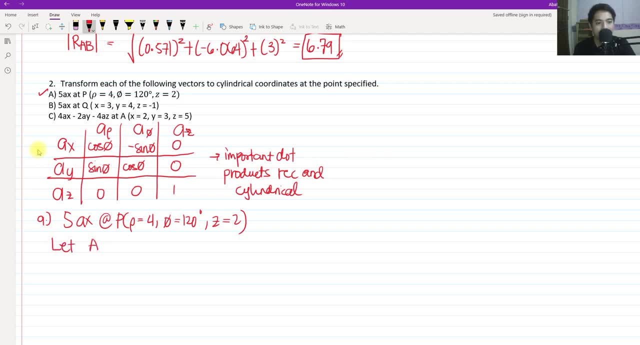 to let. okay, a as our 5ax vector 5ax. so what are we going to do is to get the components of a in terms of uh row, because we are trying to find the cylindrical coordinates of this vector at the point row phi and z. so we have a sub row, then we have a sub phi and then we have a. 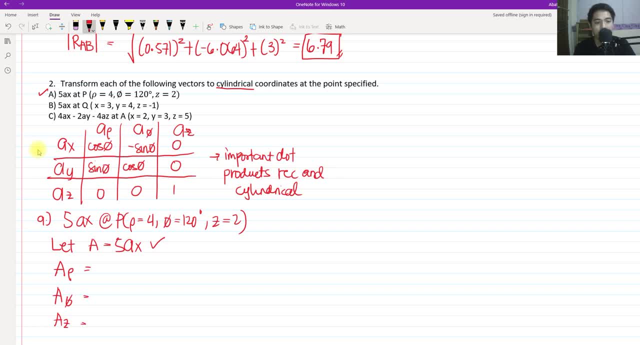 sub z. Okay. Okay, using this, what are we going to do is to have- we're going to get the dot product of a and then a unit vector. okay, a sub phi. okay, a sub rho, and this one, also a, dotted by a sub phi. 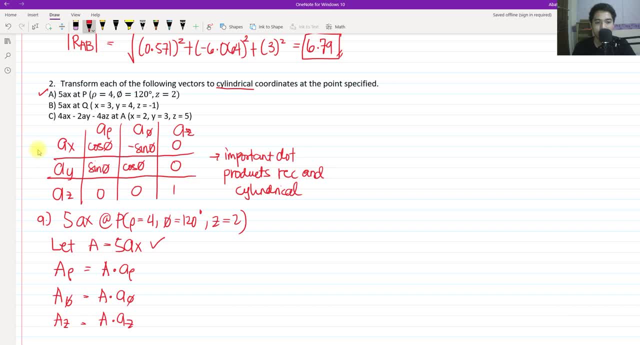 then a dotted by a sub z. so that is dot product, not multiplication. so the essence is that, okay, of this table, of this table above, is that if we get the dot product of ax and, for example, a sub x and a sub rho, we need to evaluate the cosine of phi. okay, so what we're going to do is: 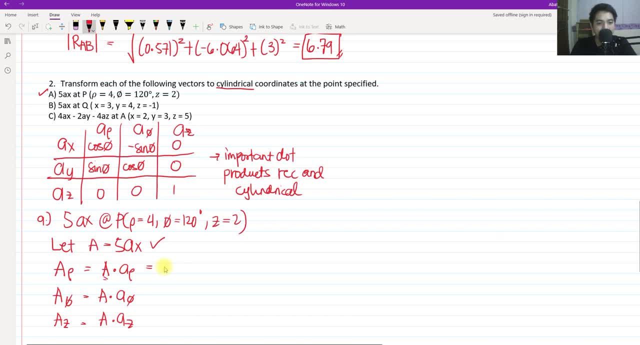 that we have. since a is 5ax, that should be dotted by a sub rho, and since a is 5ax here, that this should be dotted by a sub phi, and since we have 5ax here all again, and then we, that is dotted by a sub z. so what happens is that: 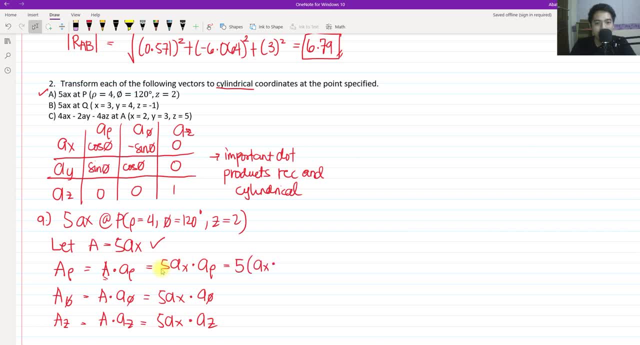 we have 5 a sub x dotted by a sub phi- okay. and then we have 5, also a sub x dotted by a sub phi. we have 5 a sub x dot product by a sub z. we just factored out the 5, okay. so what's the essence of? 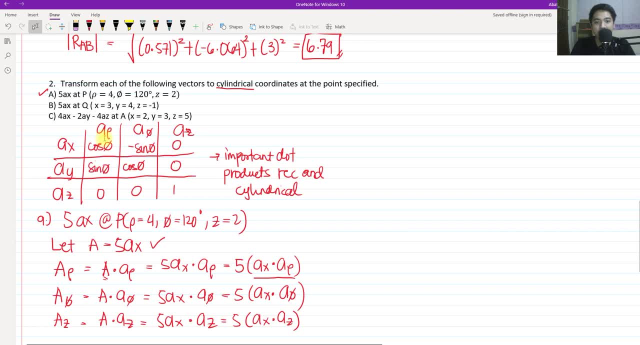 this. so that's where the table gets into work. so we have a sub x dotted by a sub phi or a sub rho. i mean that would be 5 cosine of phi because of the table here. oh, and for letter, uh, for our phi. okay, so we have 5, a sub x multiplied by a sub phi, and that is what negative sine. 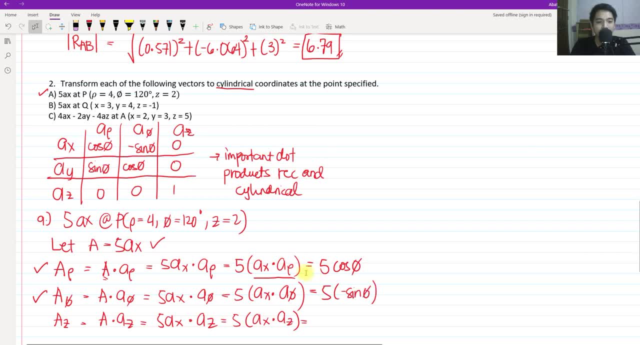 of phi. and of course, for the last one, we have a sub x multiplied by a sub z, as you can see here, dotted by ax and dot product by a z. that should be zero. so what would be the value of phi cosine? that would be the value of the given points here, the phi of the given point, that is, 120 degrees. 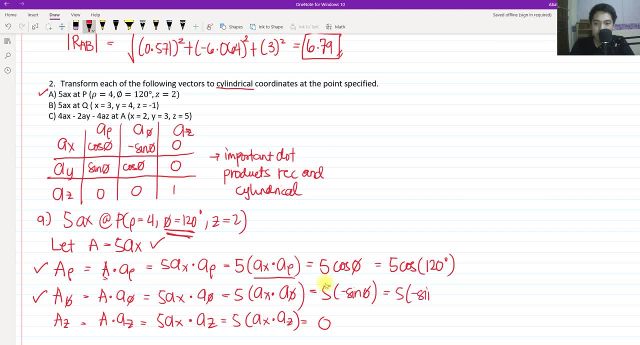 here we have five negative sine. this is still a negative sine of phi. so we have 5 cosine of phi, so we have 120 degrees also and of course this would be zero. so upon evaluating 5 cosine of 20, 120 degrees, that's negative 2.5. okay, so meaning this is the phi or this is the rho. 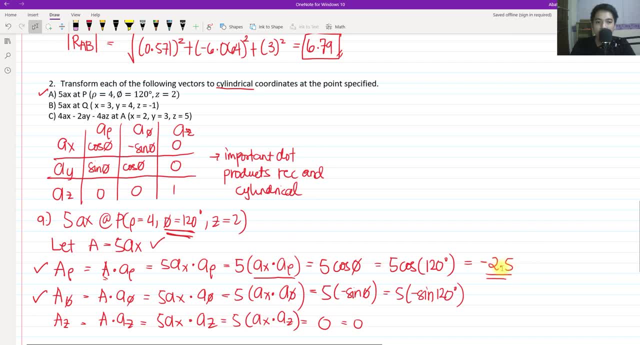 in terms of cylindrical coordinates up of the 0.5 ax at this point. okay, so evaluating a sub phi, we have what, if you input it into our calculator? we have negative 4.33 and of course the a sub z is zero. hence the point okay of the vector a in terms of, for example, that vector a is our answer. 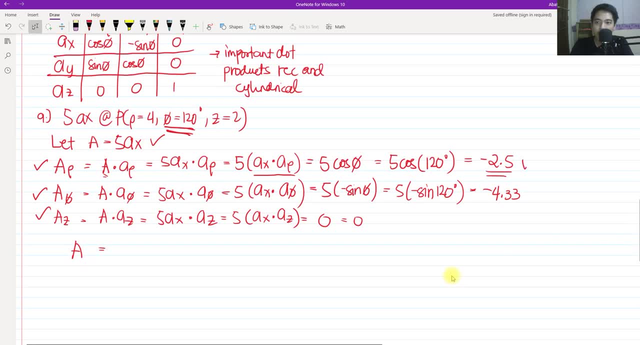 okay, is what? these are the components of the rho, phi and z. okay, that's the components. so we have negative 2.5 a sub rho, then minus 4.33 a sub phi. so this is now the transform of that 5 ax at this point, okay. 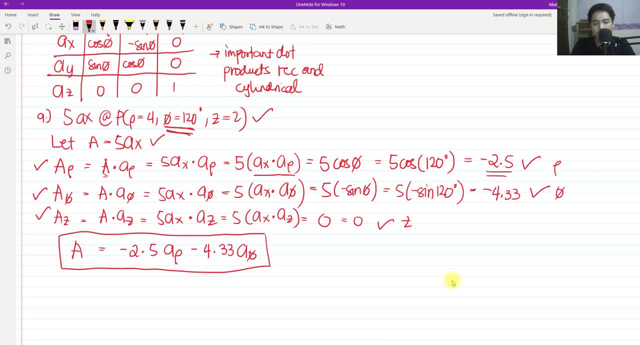 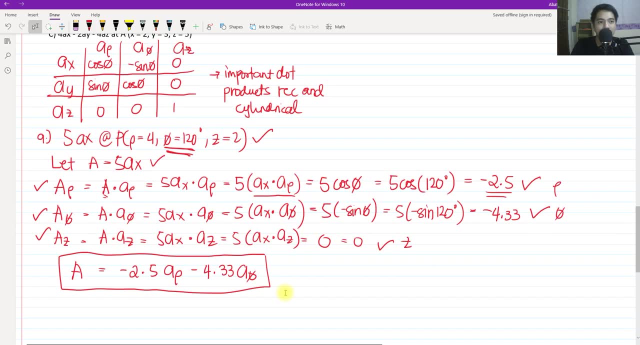 at this given point. cylindrical coordinates. i hope you get that. that's the purpose of having this. dot products: okay, table of dot products. so for letter b: so we have 5 ax at q equals x. so we have 5 ax at x. at q, let's say q, okay. at q, x equals 3. then we have: 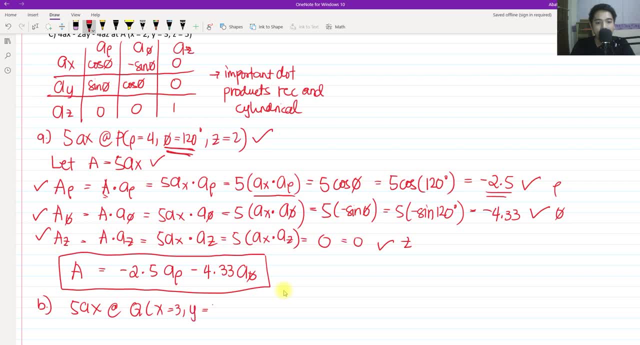 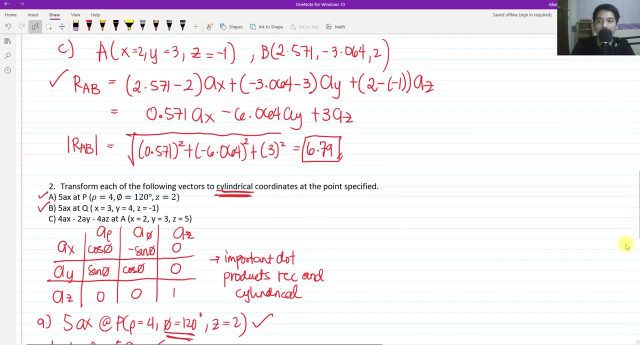 y equals 4, and then we have z equals what is that? negative 1? so, as you can see, here the question is actually asking us: what is the function of z and what is the function of z? and z equals 3, and so that's where z comes in and z follows the lambda. so we have z and z equals 4. 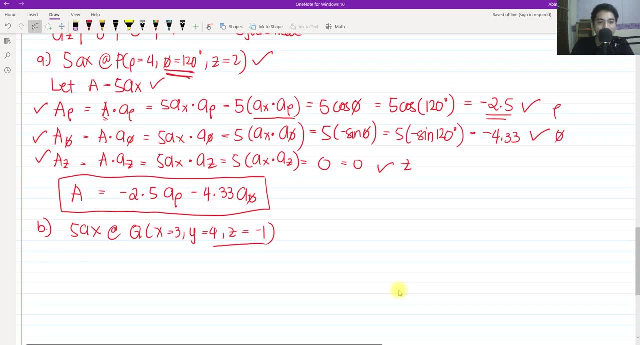 and z equals 5, z equals 5, and so we have z equals 4 and z equals 5, and z equals 5 and z equals 6 in this case. we have 0.5. x would be the octan, so we have z equals 6 in this case. and then we have a. 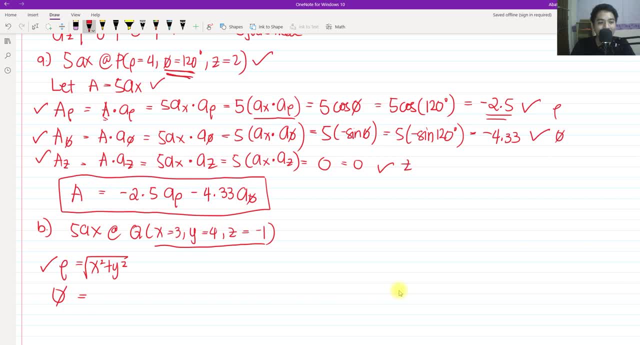 root of z equals 3, z equals 3, so all right. so for the question: what is the function of z and z? okay, and this is what we have to do, we have a square root of z equals 3, so we could now just use the constant of z and z equals 3, and in this case, it's going to be the product of z equals 4. so 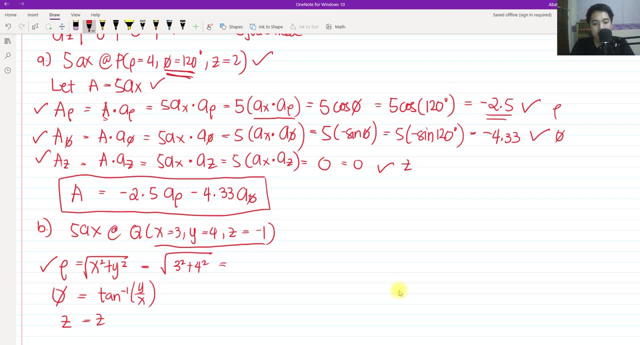 squared plus four squared, then we have a five. okay, and this should be arc tan of four over three. that's y all over x. that is 53.13 degrees if you try it in your calculator. so z is still negative one. so the point q, in terms of cylindrical coordinates, would be five. okay, we have 53.13. 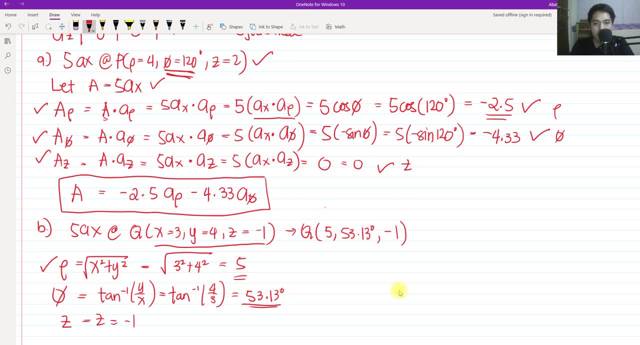 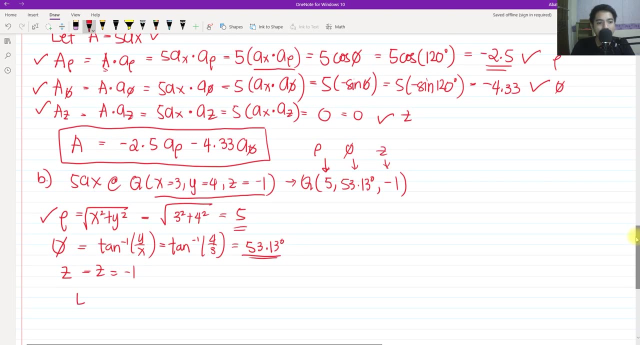 degrees and then we have negative one. so this would be our rho, this would be our phi and this would be our z. so again, following a while ago, the, the process we are going to let what a equals five ax so that we have to get a. what a phi, sub phi. 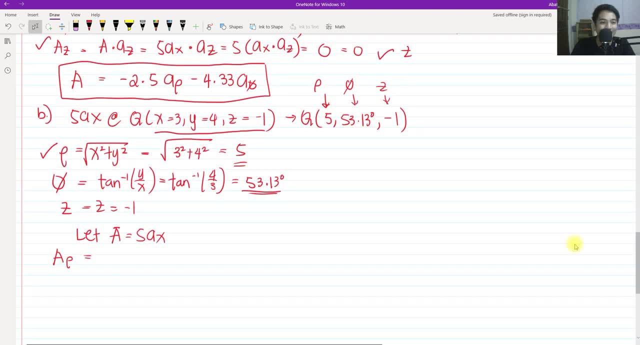 then we we're going uh, a sub rho, i mean, and then we have a sub phi and a sub z, using again the dot product. so we have five. we have ax dotted by a- what unit vector? a sub phi. so we have five. a x dotted by a sub phi, this is raw. i'm always uh, i'm always confused. no, it's always raw, this is. 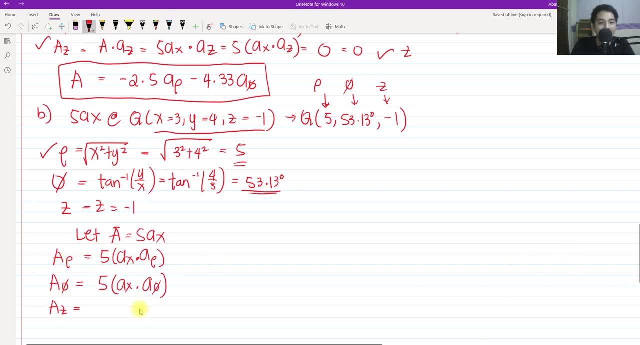 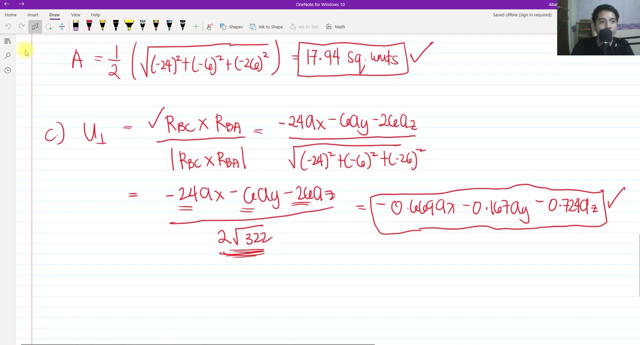 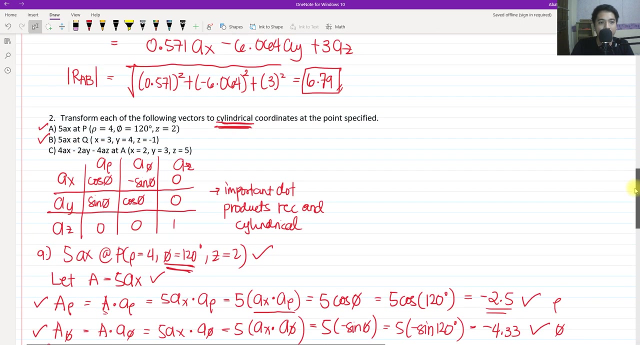 okay, please forgive me, this is raw, this is phi. so we have five a x multiplied or dot product, product by a sub say okay, so you see if we are going to go back in our uh- oops, we are going to go back in our uh table. so we have ax dotted by a sub, rho would be cosine. okay, cosine would be cosine. 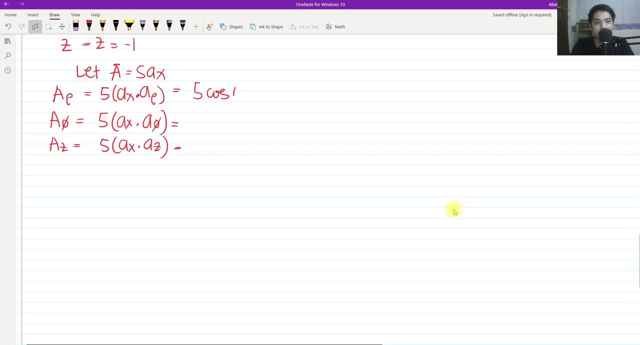 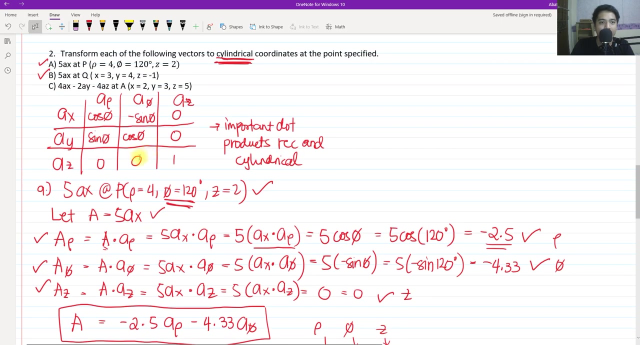 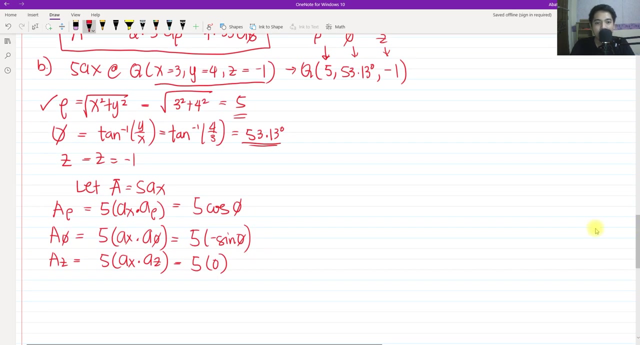 of phi. so this would be five cosine of phi. this would be five negative sine of phi a while ago, and this would be five multiplied by zero. okay, so, as you can see, a sub x and a sub z, when we dot product, they them, we have get zero. so five times zero would be zero. so again, so we have five cosine. 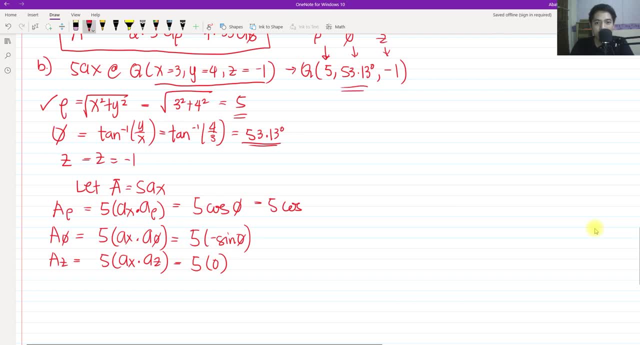 the phi now is actually 53.13, 53.13. so we have 53.13, and then we have five multiplied by negative sine of 53.13 degrees. then we have zero here. so, evaluating this in our calculator, we have three for a sub phi. we have 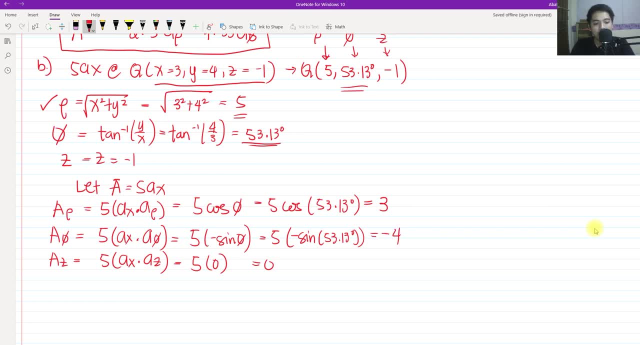 negative four, and then we have zero. so hence, okay, hence the point five: a x at the point q here. q here, in terms of cylindrical coordinates, should be three, a sub rho, okay, and then we have minus four, a sub phi. so that would be the the answer. okay, if we are going to transform. 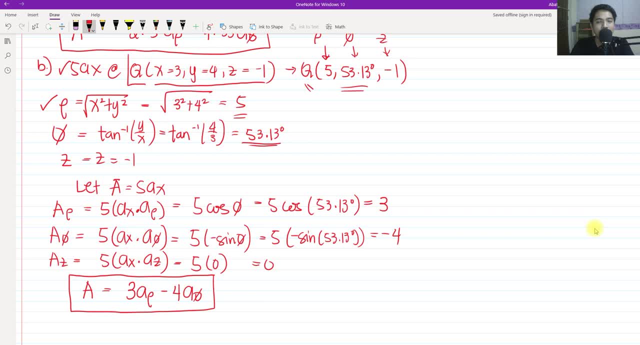 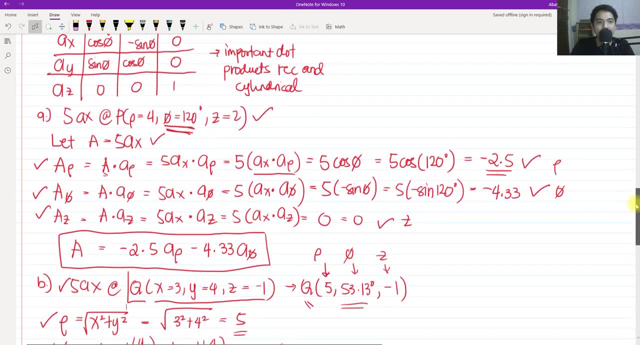 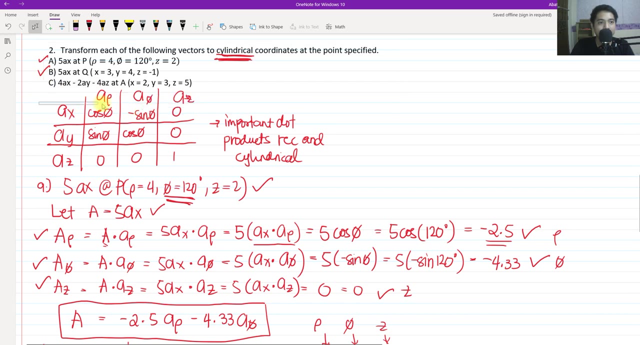 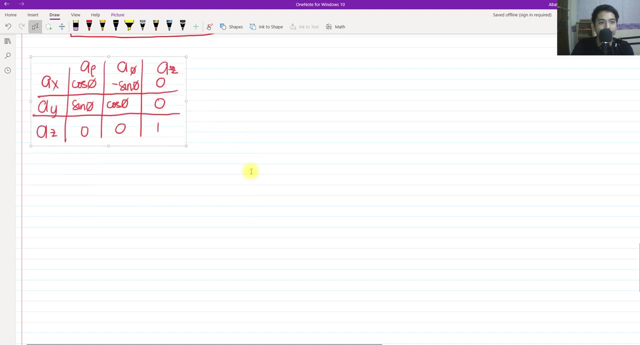 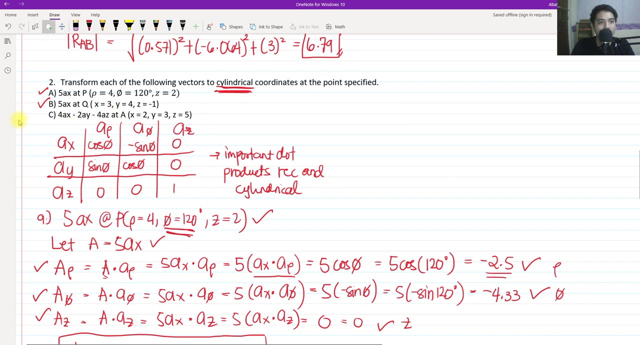 five a x at this point, q in terms of cylindrical coordinates. okay, so let me just copy this first. copy the table. oops, okay, let's just copy that table for our point of reference. okay, So for number, you have files three. transform the four a x. transform the four a x in terms of cylinders. правильно yang r. 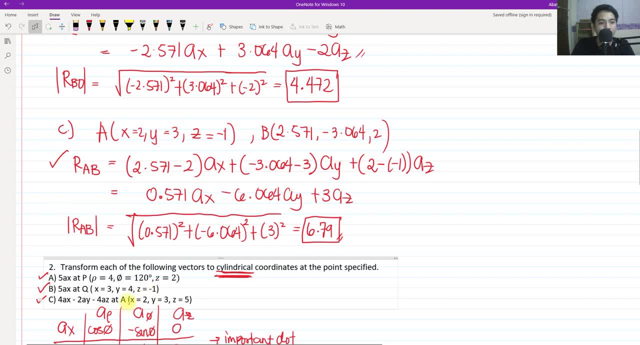 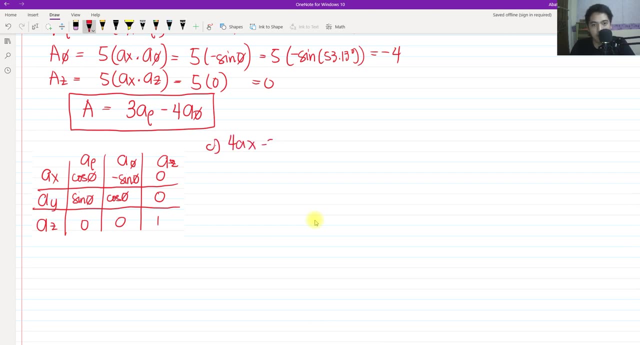 minus 2 ay and minus 4 az. at point a, x equals 2, y equals 3, z equals 5, of course in terms of cylindrical. okay. so we have for letter C, we have 4 ax minus 2 ay, minus 4 az. at what a equals x equals 2, y equals 3 and z equals 5. so this is a little bit. 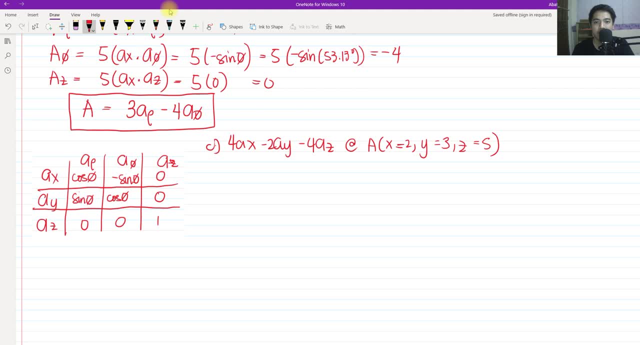 long in terms of solution. so the first thing that we're going to do is to convert a in terms of cylindrical coordinates. so if we convert that, that would be 2 squared plus 3 squared, that is 3.61. so we have the phi, we have the arc tan of y all over x. 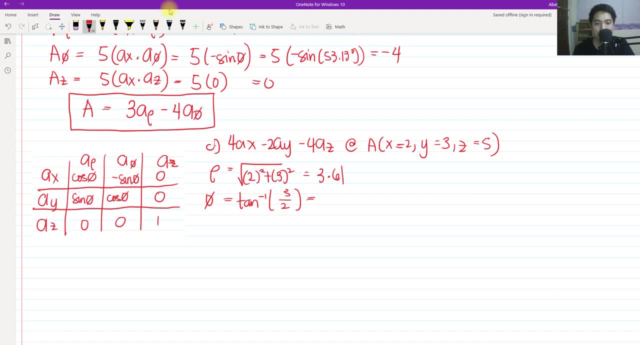 that is 3 halves, so we get 56.31 degrees. and for the z that's equal to 5, so we have now the points a in terms of cylindrical, so we have 2, 3.61, so we have phi equals 56.61. 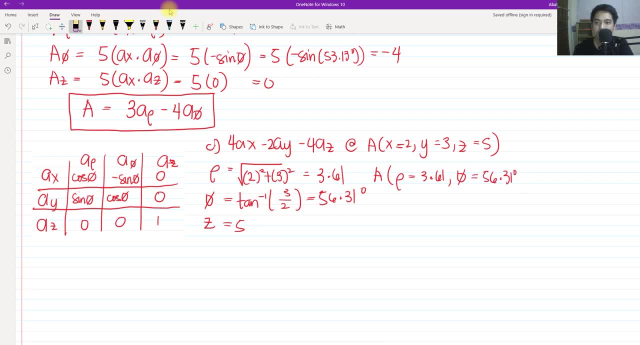 degrees and then we have z equals 5. okay, so now we can perform. so we are going to let a equals 4 ax minus 2 ay minus 4 az, and then we're going to get again the a row sub row, a sub phi and a sub. 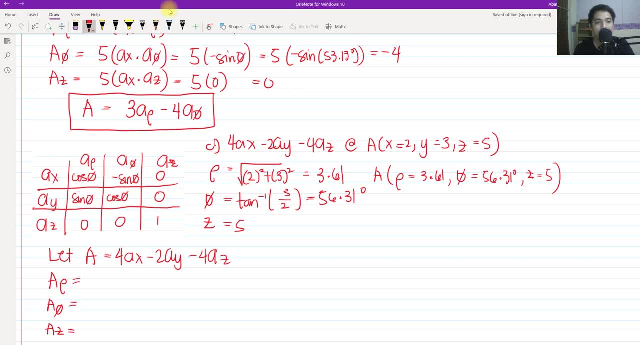 say: okay, of that. so we have what. we have a dotted by a unit vector of a sub row. we have a dotted by a unit vector of a sub phi. we have the a dotted by a unit vector of a sub say. so what are we going to do with that? of course, 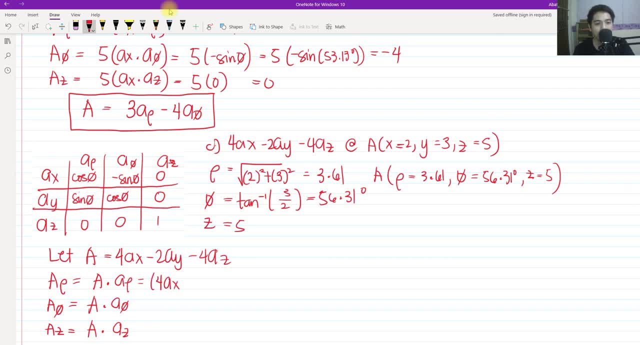 we have 4 ax minus 2 ay, minus 4 az, and then dotted by a sub row. okay, so that is how we do that. so this would result into 4 ax dotted by a row, minus 2 a sub y dotted by a row, minus 4 a sub z dotted by a row. okay, so again we have here our values for the dot product of: 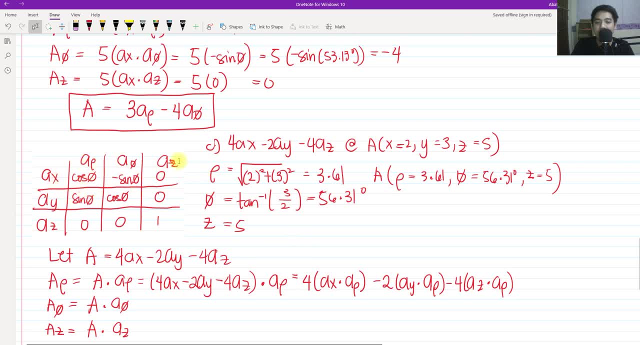 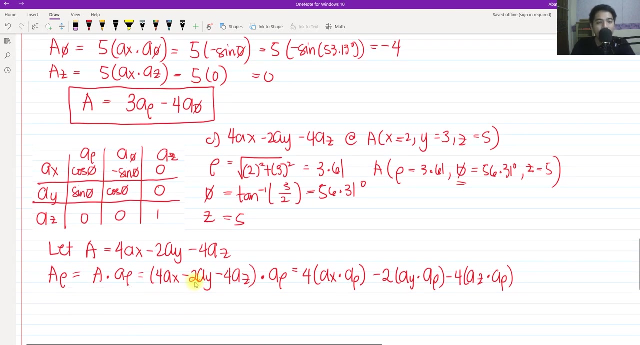 different rectangular coordinates and the cylindrical coordinates. so this is what we are going to refer to, okay, and we're going to use the values of the phi here, okay, for our calculations, okay. so let me just erase this first. let me just erase this first and we focus on a sub. 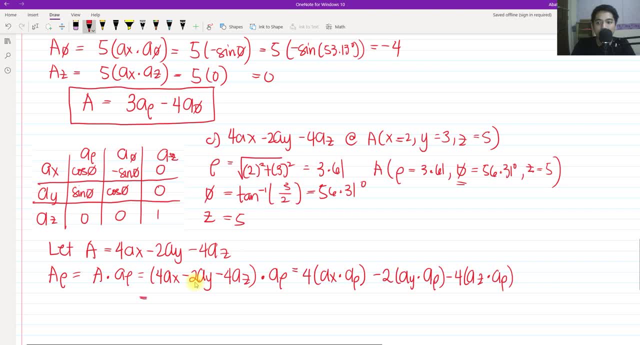 rho. so we have what we now have: four: that product by a sub x and a sub rho. that would be cos sine of phi minus two. that product of a sub y and then a sub rho would be sine of phi minus four. that product of a sub z and a sub. 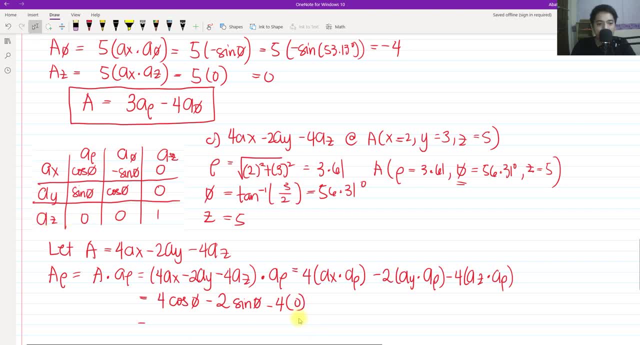 rho, okay, would be 0, so this would be 4 cosine. the phi here is the phi that we have solved a while ago, so we have 56.31 degrees minus 2 sine of 56, 56, I mean, I'm sorry. so this would be 56.31 degrees 2 sine of 56 minus 31 degrees minus 0 of. 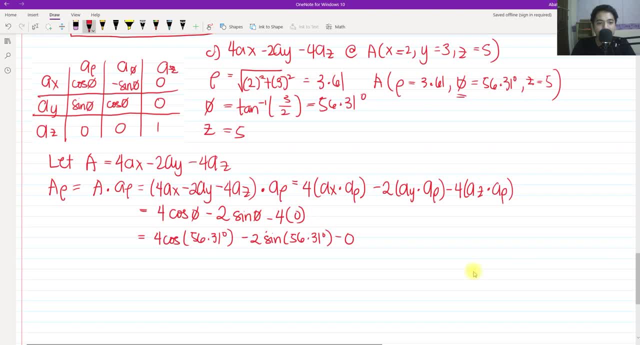 course, because 4 times 0 would be 0. so if we evaluate this, okay, so our answer that we would get would be 0.555. that's only the, the term or the scalar quantity of the a sub Rho. okay, so let's try a sub phi, and again, that is a that. 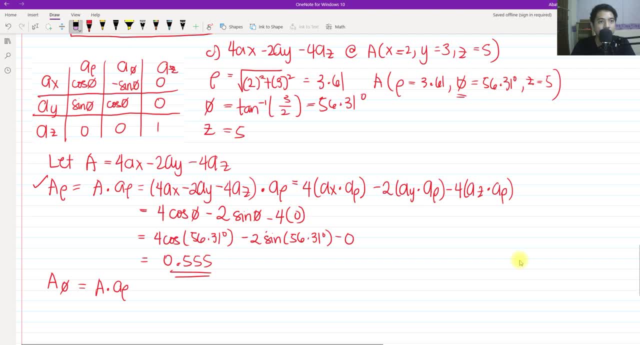 product by a unit vector, a sub V. let me just rewrite this below: so we have a sub V, that we have a dotted by a sub V, so that becomes 4 a X minus 2 a Y minus 4 a Z dotted by a sub V. so what will happen is that we have 4 a sub X dotted by a sub. 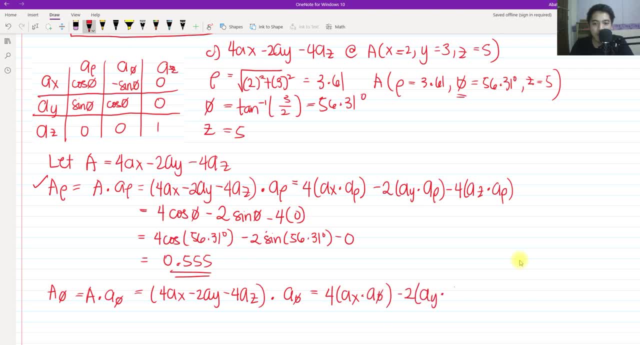 V minus 2 a sub Y dotted by a sub V and then minus 4 a sub Z dotted by a sub V. so refer to the table for the dot product. so we have 4 a X, a sub X and then a sub V. would be negative sine of V. 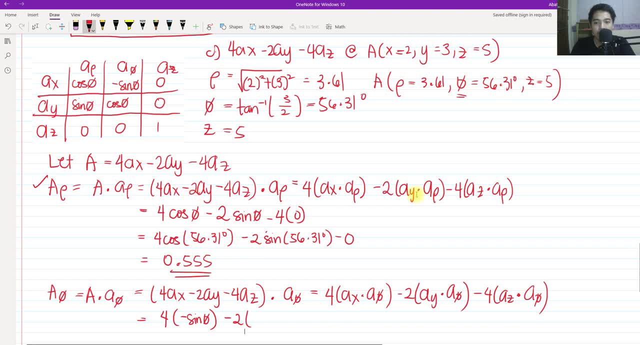 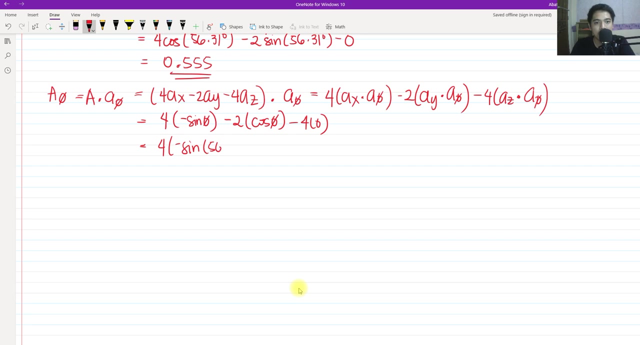 okay, then we have minus 2, a sub Y, and then what a sub V is cosine phi on the table minus, we have a sub c dotted by a sub phi. so that is still 0 minus 4 times 0. so we need to evaluate. we have 4 negative sine of 56.31 degrees minus 2 cosine of 56.31 degrees minus 0. so upon 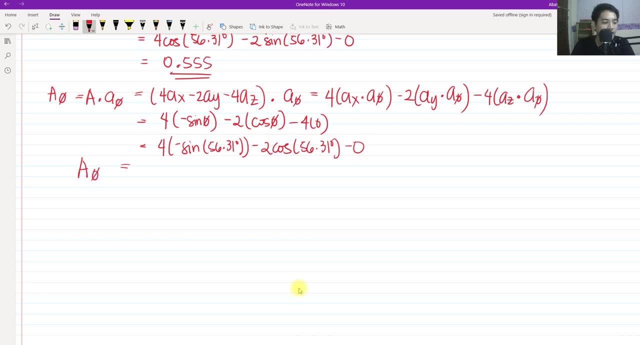 evaluating we we get the component of a sub phi and that becomes negative 4.44. that's a component. and lastly, for a sub z, we have that product of vector a and the unit vector a sub z. so we have 4a sub x minus 2ay minus 4a sub z dotted by unit vector a sub z. that becomes: 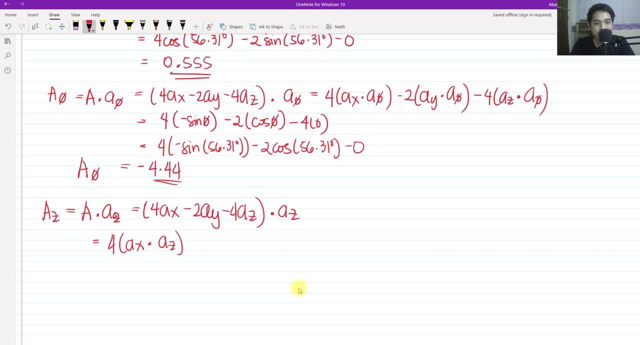 4a sub x minus 2ay minus 4a sub z dotted by unit vector a sub z, that becomes 4a sub x minus 2ay. 4 a sub x dotted by a sub z minus 2 a sub y dotted by a sub z minus 4 a sub z dotted by a sub z. 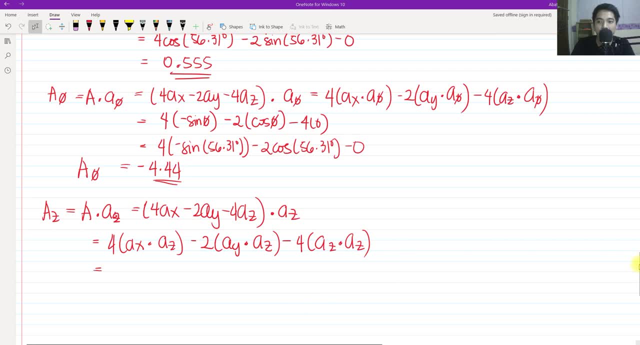 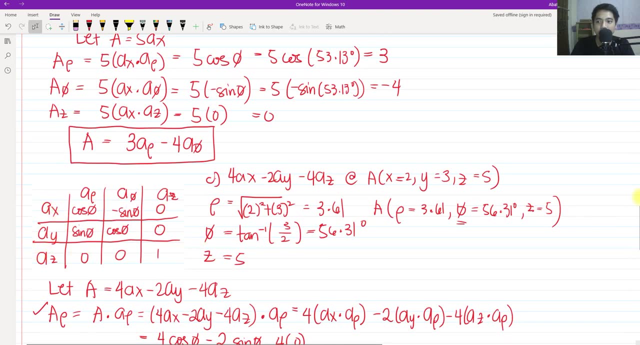 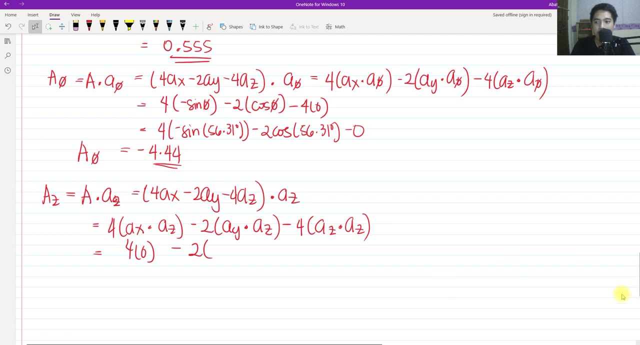 So, referring again to our table, so we have a sub x dotted by a sub z. So we have a sub x dotted by a sub z would be 0.. Okay, that would be 0. So, 4 times 0 minus 2, a sub y dotted by a sub z. a sub y dotted by a sub z is 0.. 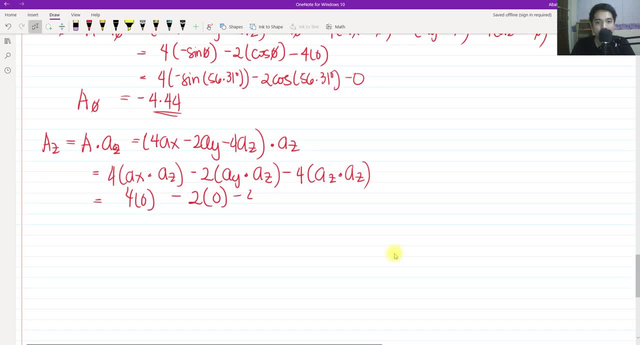 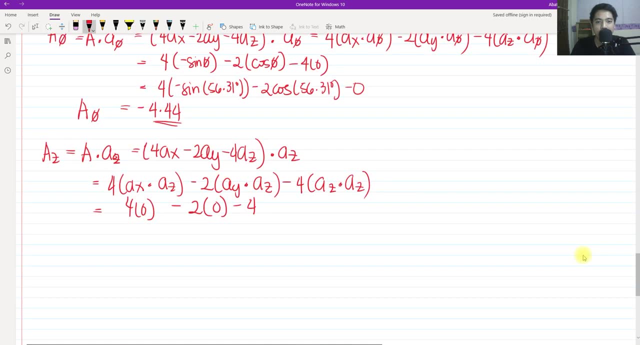 That would be 0. also, Minus 4, a sub z dotted by itself, That product dotted by itself, is 1.. So we have, so we all know it's obvious: 4 times 0 is 0, minus 2 times 0 is 0.. 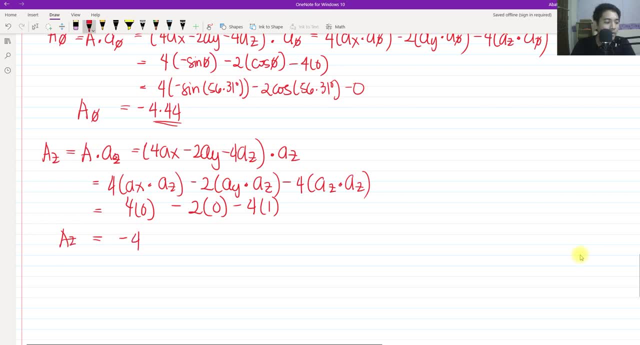 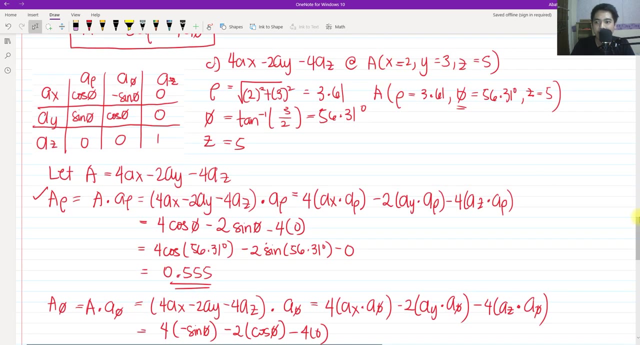 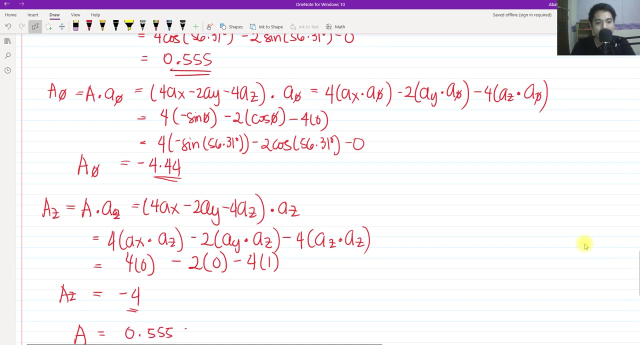 So our a sub z would be negative 4.. So our answer hence for this formula is that the cylindrical coordinates of that point at that specified point, okay, at that specified point a, here would be what Negative? or 0.555, that's the component of a rho, a sub rho. 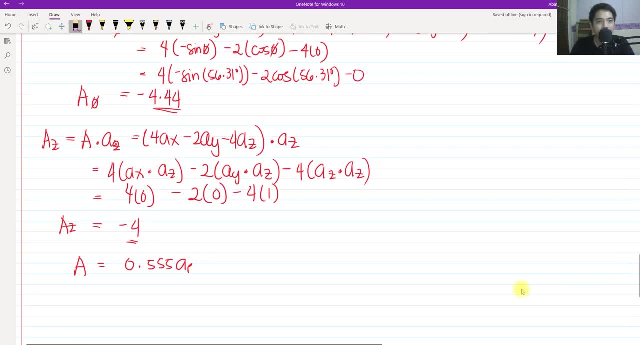 And then we have: this is a sub rho. Let me just rewrite A sub rho minus. we have 4.44 a sub phi. then we have 4 minus 4 a sub z. Okay, so this would be our answer. 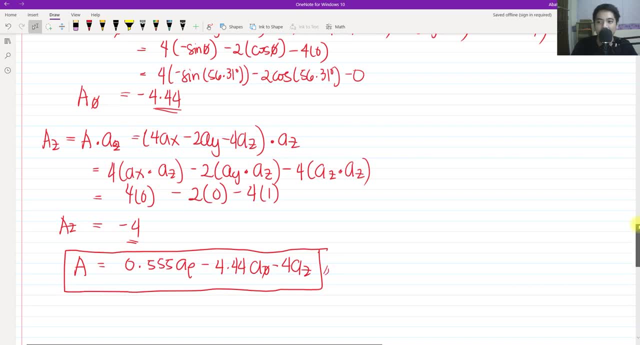 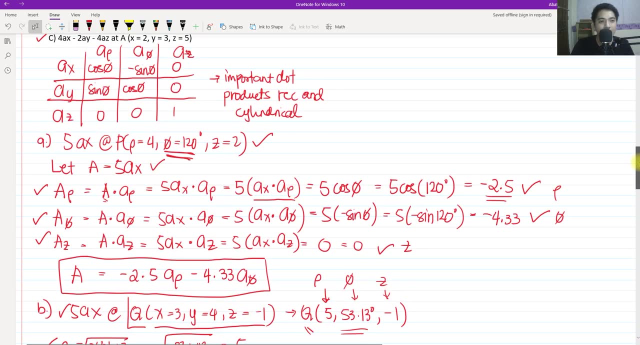 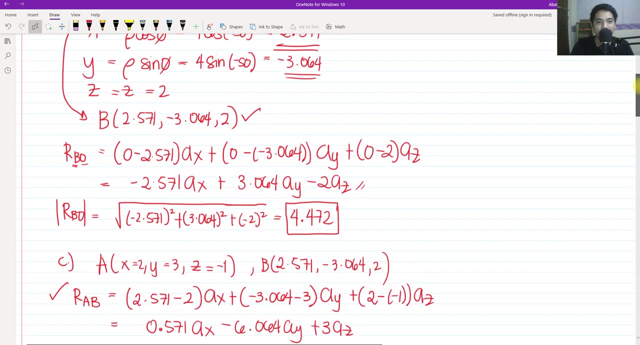 Okay, guys, I hope you learned something new about our topic. all about the cylindrical coordinates and how we convert those cylindrical coordinates into rectangular and vice versa, and how we get a specified Vector at that specified point. okay, in terms of cylindrical coordinates. 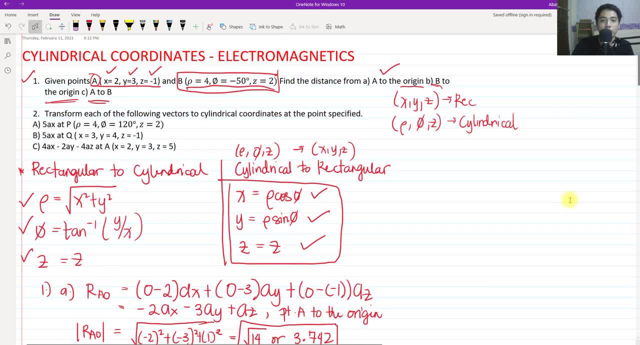 So if you find this video helpful, please don't forget to subscribe, and if you are new to my channel, please see my other videos about electromagnetics and other math and engineering courses. So thank you so much for listening. Again, this is Inger Abad. God bless you. 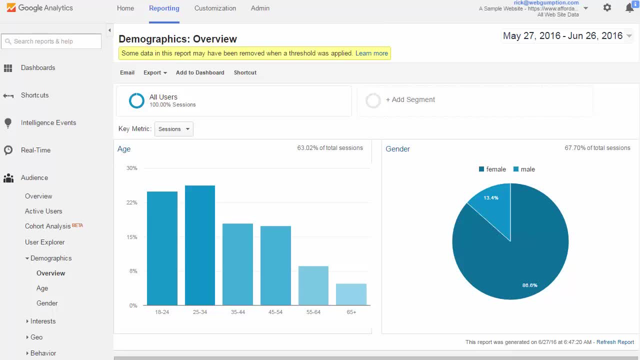 Demographic Overview Report. Demographic Overview Report gives us a high-level view of age and gender metrics on our website. So to access this report you're going to go left-nav- audience, demographics and then overview. So this overview report, it's a very high-level view of the different age groups and genders on our websites. 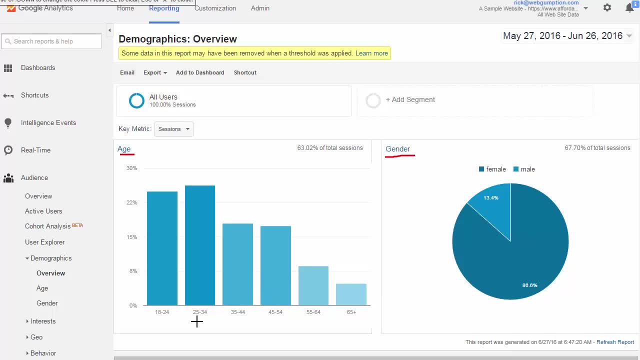 And Google Analytics breaks our age groups into about six different groups And from this chart we can see the 25- to 34-year-olds are the most common age group, whereas 65-plus are the least common And, on the gender side of things, we note that females account for about 86% of its traffic. 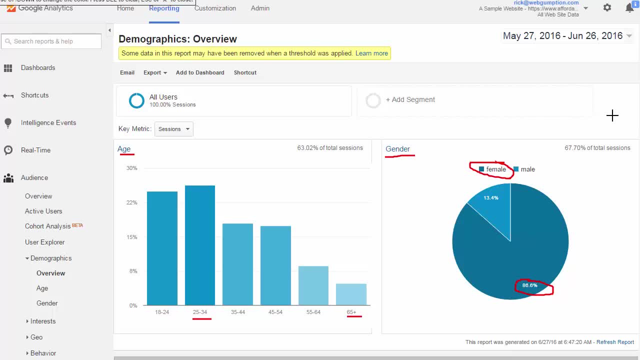 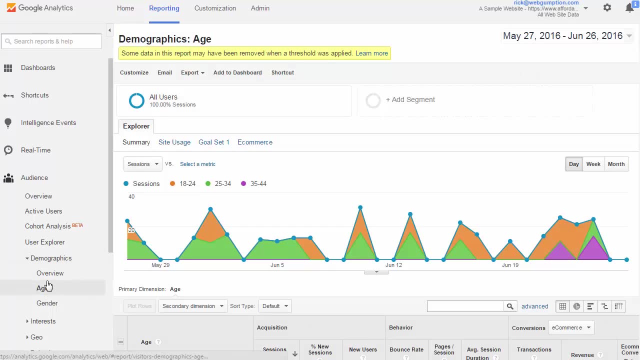 Not a surprise, We're a makeup website. To get more details on each, we're going to jump into the specific age and gender reports, The Demographics Age Report. So the Demographics Age Report breaks down all of the different age groups and specific metrics, including traffic, behavioral and conversion metrics. 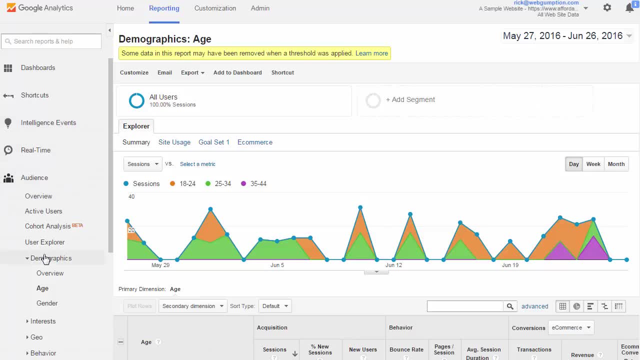 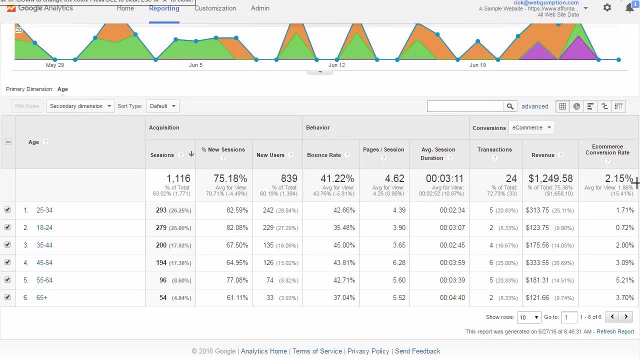 To access this report, you're going to go left-nav audience: demographics and age. Some things we'll see on the age report are that we break our age groups down into about six different groups And we get our basic traffic, behavioral and conversion data on each. 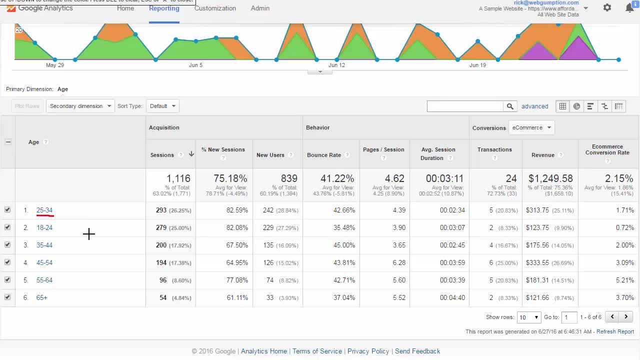 So let's take a look at the age group 25-34.. This is our most common age group. we can see About 293 vehicles And that's about 26% of our site traffic. Again, we get information, including like bounce rate and pages a session for this particular age range.